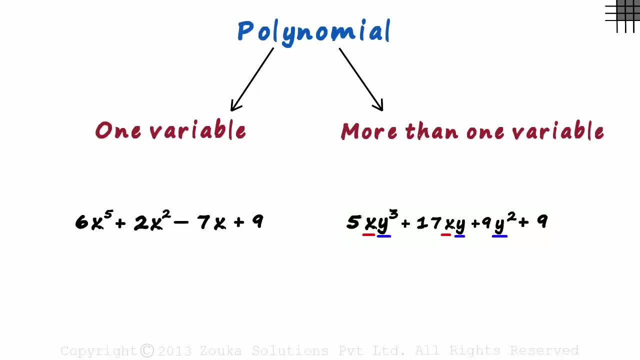 This has two variables, x and y, which makes it fall into the second category. So what about these two categories? Why did we form them? It is for the concept. we will look at in this video: The degree of the polynomial In the first category, where we have just one variable. 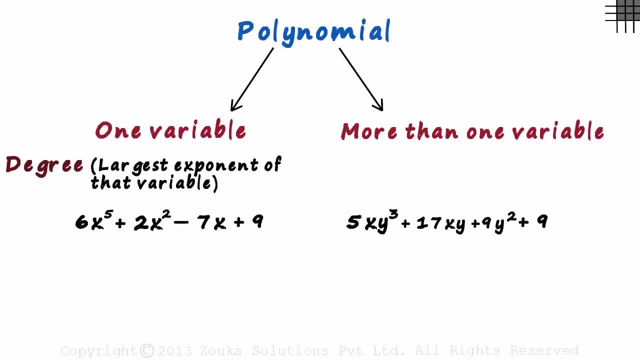 the degree is the largest exponent of that variable. Here, 5 is the largest exponent, which tells us that the degree is 5.. The degree of this polynomial is 5.. Let's look at a second example in this category: 21x plus 6x cubed. 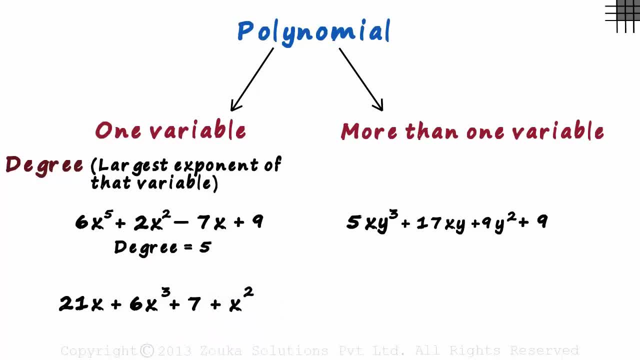 21x plus 6x cubed plus 7 plus x squared. In the first term the degree of x is 1.. In the second term, the degree of x is 3.. And in the last term it's 2.. 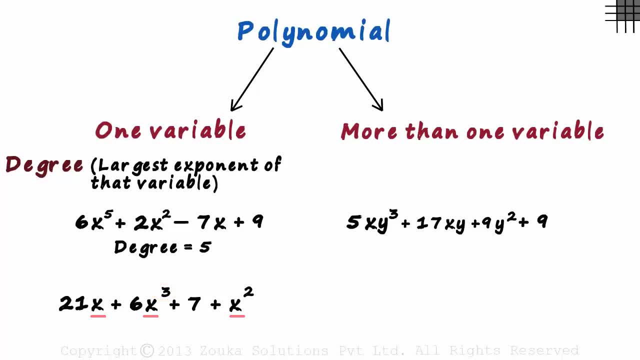 3 becomes the largest exponent of the variable, And that's why the degree of this polynomial is 3.. Is it any different in the second case? Yes, slightly different In the second case. for each term we add the exponents of each variable in it. 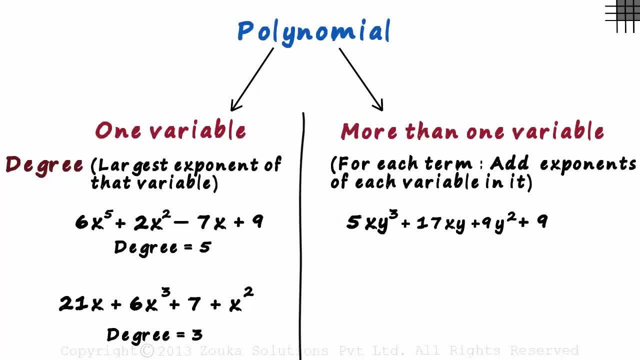 How will it work out? for the first example? Remember we have to look at each term individually. Consider the first term, 5xy cubed. We had to add the exponents of each variable. in it, The exponent of x is 1 and the exponent of y is 3.. 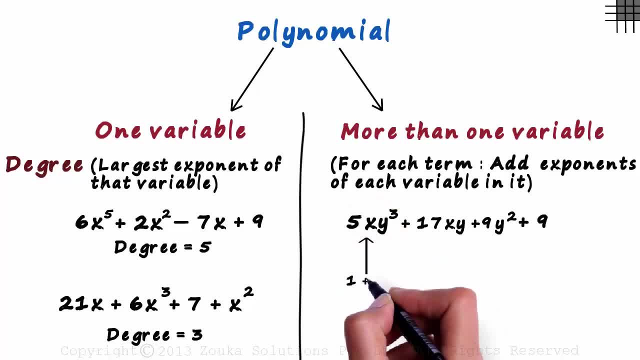 So for the first term, we consider the power to be 1 plus 3, which is 4.. Now we come to the second term. There are two variables, x and y, and each of them have an exponent equal to 1.. 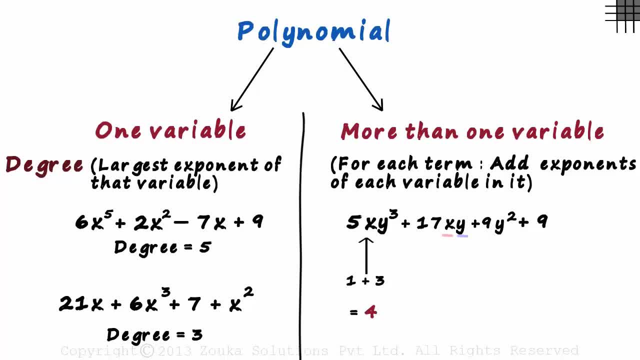 Adding the exponents, we consider the exponent of this term to be 1 plus 1, which equals 2.. In the third term, we have just one variable. Its exponent will just be 2.. And as we have no variables in the last term,